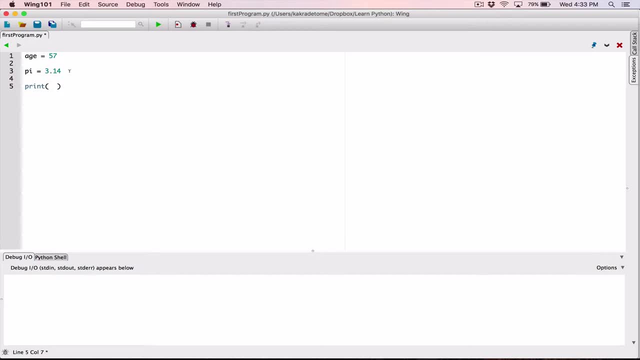 But remember, we talked about it briefly and said that a function is basically one or more lines of Python code wrapped up together and then given a name. And when you install Python, okay, Python in itself the programming language, Python. the people who developed that language, you know, created some functions for you because they didn't want you to, you know, redo it. There are some basic functions that we would need. For example, if we wanted to display something on the screen, they wrote the print function for us. 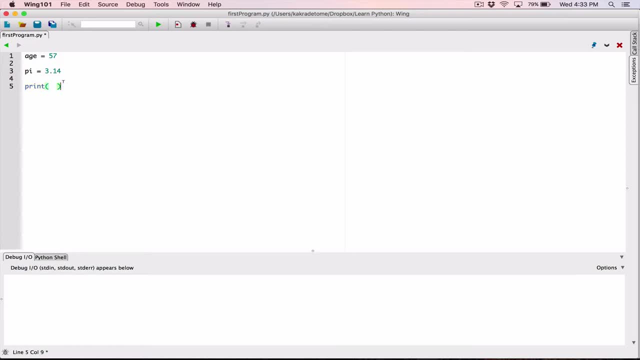 We don't have to rewrite it ourselves. And so they put together some lines of code- one or more lines of code, I don't know how many lines- And they gave it a name. well, and they- sorry, they wrapped it up together and then they gave it a name print And anytime you use a name it's really called. 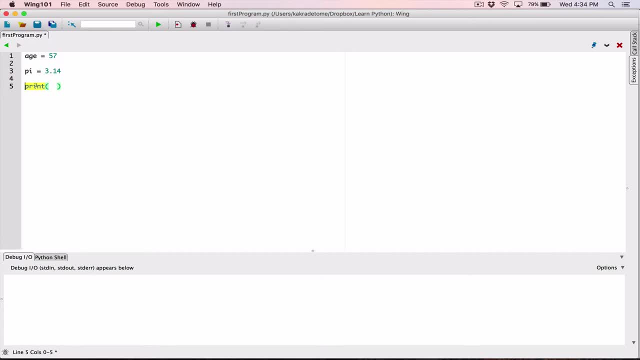 I'm calling the name Anytime you type the name any time you call. that functions okay. that's when you just use it. referred to the name Any time you call it. it's going to ask you: what do you want me to print? 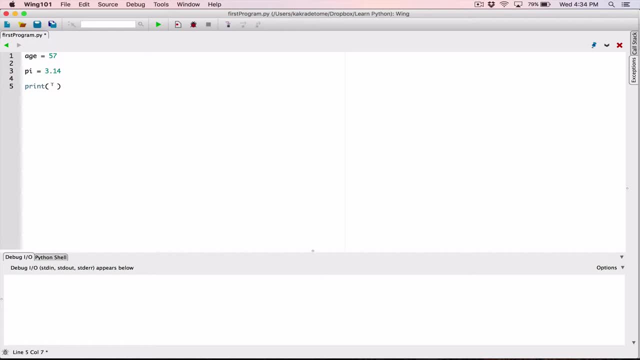 And that's what you provide in these parenthesis, in this parent, in this parenthesis, Right? So when you provide that value, which is really called an argument, that value is called an argument. So when you provide that argument, it's going to display that argument. whatever you give it On the screen, it's going to display it on the screen. 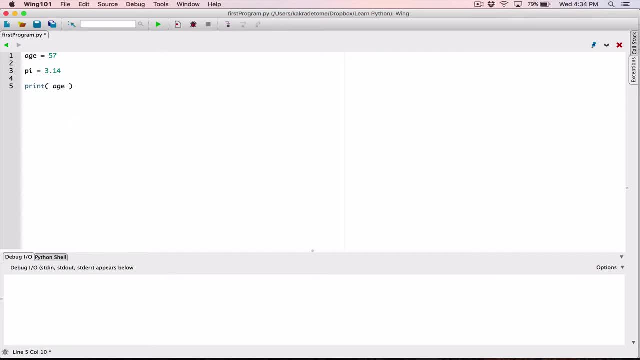 So In this case I wanted to display the content of age. When I run it, it's going to display 57, right. Same thing: when I display the content of pi, it's going to display 3.14.. All right. so over here we said this is an int and this is a float. 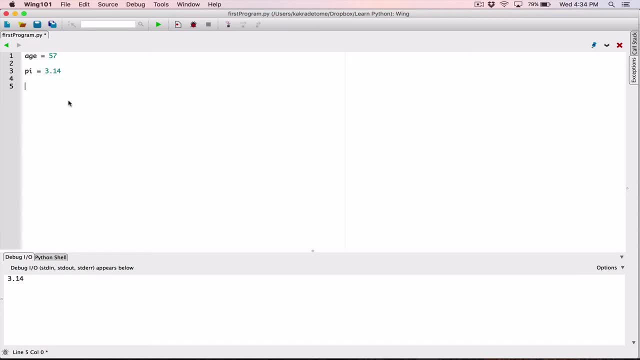 What if we didn't know? There's another function that the people who created the Python language created for us, and that function is called type, And type will basically tell you the type of data, of a value that you give it right. So let's switch to the Python shell. 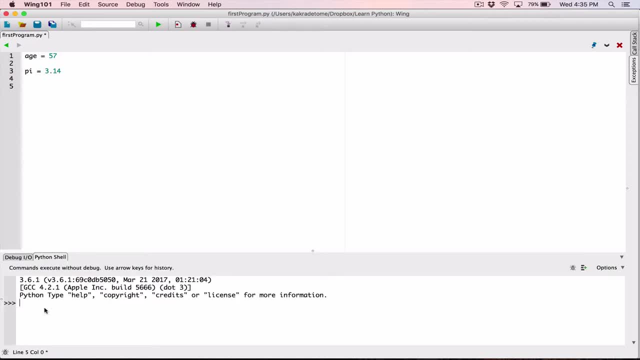 Remember we said the Python shell is an interactions pane. It's basically testing out simple lines of code, or a few lines of code, just to see, even before you write it in your program Over here. you don't have to save the file. You can just type in a line and it will automatically give you the result. 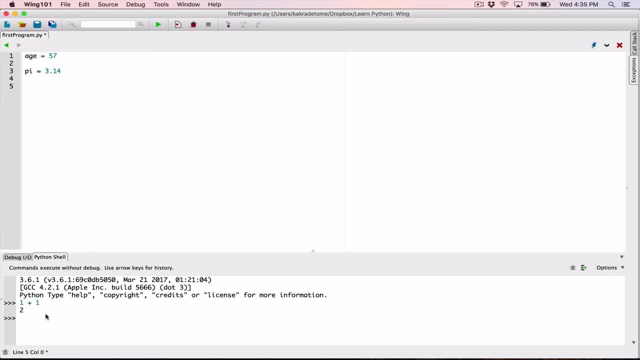 You can type in 1, what's 1 plus 1, hit enter and it's like an interaction, It's like a line, It's like it's talking to you. You say something and it replies back with a response. 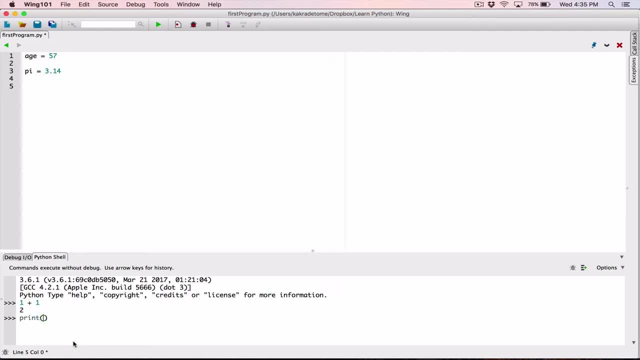 And so you can use a print function over here too and say, okay, print out. Well, over here, it wouldn't know the values over here because these are two different services. You can think of them that way. So it wouldn't really know that. okay, age has been defined with a value of 57.. 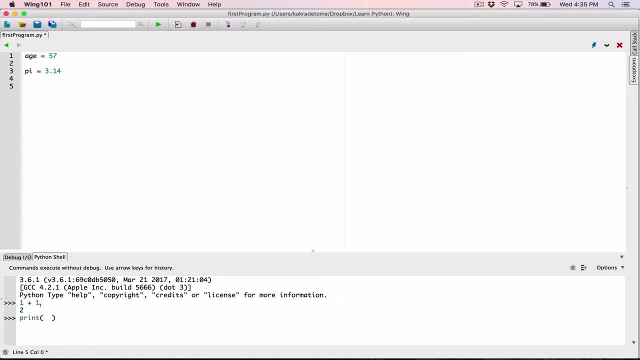 This is when we are working in the script mode, right? So this is something different, right, separate, kind of separate. But I can say something like print the value 57. I can say print out 34, or the number 34 on the screen. let's see. and then the print. 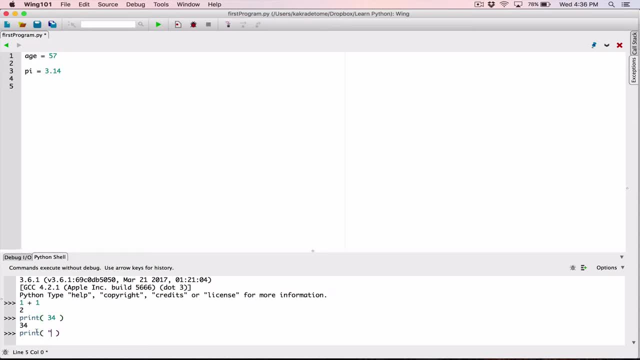 out 34.. I can say print out the value. sorry, the string cat on the screen and the print out cat. So just drag this by the ball over here, okay. So type is a function, just like the print function. You call the name. 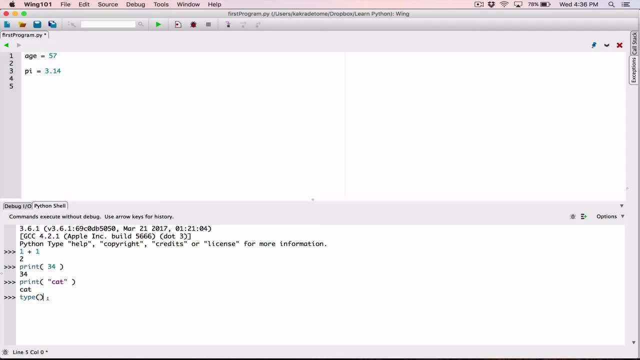 Anytime you call the name, remember functions need to have parentheses right. They either accept an argument or not. Arguments are basically what you provide in the parentheses. In this case, type will ask you: what do you want me to tell you? the type of data you? 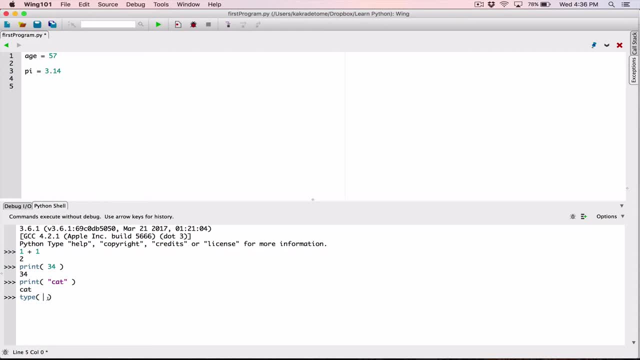 know data of. So basically, it takes an argument and tells you the type of data it is. So I'm going to ask it: tell me the type of data this is. I want to know the type of data. the number three is: 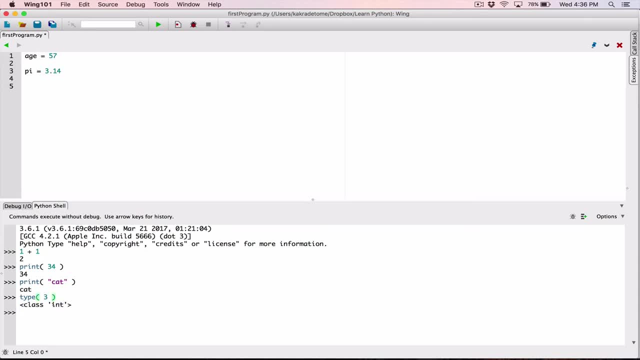 So when I hit enter, it's going to reply to me. forget about the name class here. just forget about it. I'm going to focus on what's in single quotations here. It's telling me that the number three is an int. 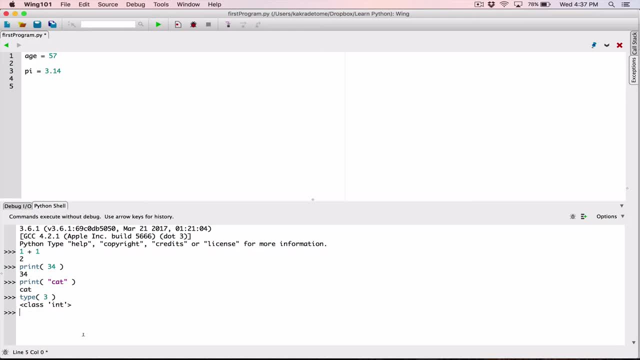 Let's try another one Type. oh, by the way, when you hit the up and down arrow key, it gives you the history of all the things you've typed. So when I'm hitting the up arrow key now, I'm hitting the down arrow key now. it's taking 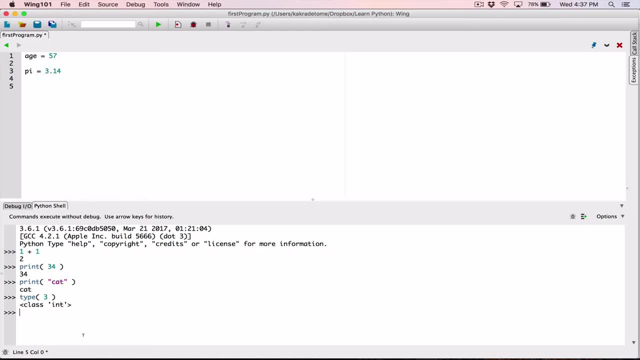 me back Up arrow key, down arrow key. All right, you can also type So type and then I can ask it: what's the type of data of this value? So 3.14.. We know this is a float, but to me we don't really know. 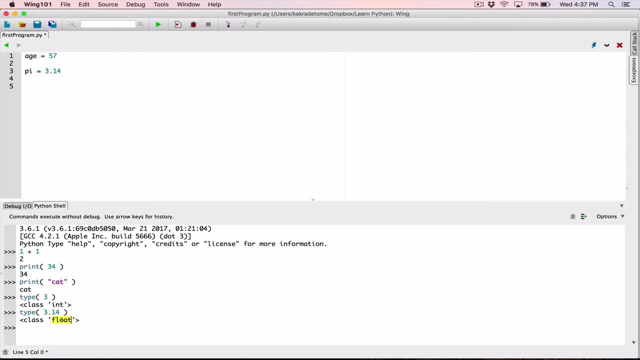 Hit enter and it comes back and it tells us this is a float Focus on just this value for now. So that's how the type function works. So the way this is working is because the people who this is working in such a way. 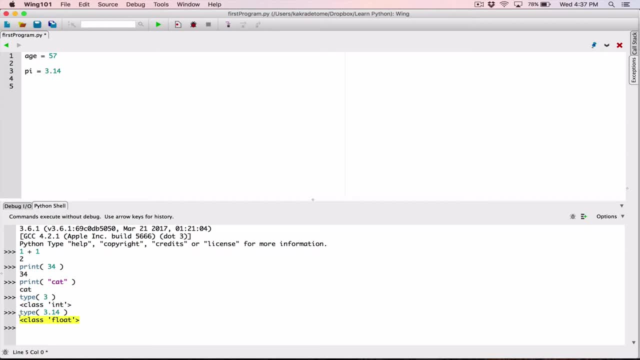 that when you give it a value, it tells you the type. The people who created the Python language created this for us, this function for us, And again we'll talk more about functions and how to create our own custom functions and how to use a predefined function. 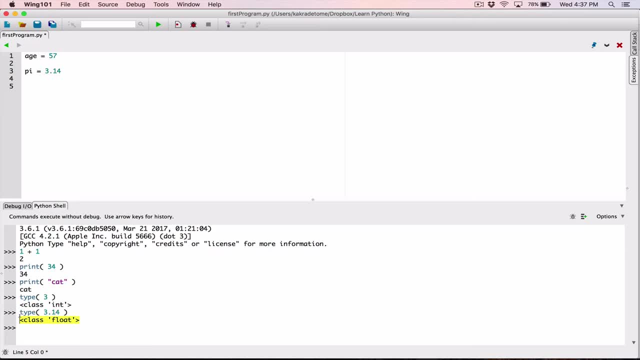 I mean we are using the predefined functions already, The functions that have already been created, So you can also use type over here in your code. There's a slight difference When I use type. okay, the type of, let's say, the value stored in age. 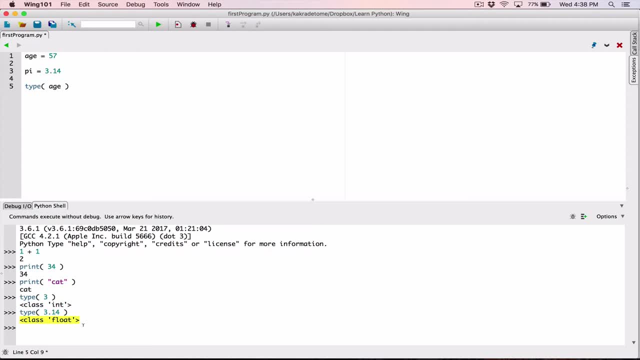 Now type over here in interactions pane. well, it's telling us over here, it's showing us, it's printing us, printing to us the value, The type of data that value is. That's because that's how the Python shell is designed to tell you to automatically. 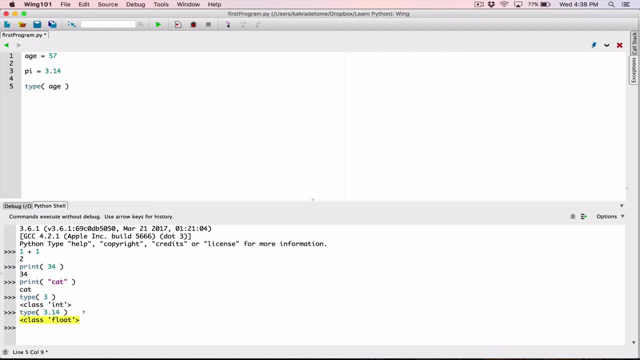 print to you the result without even without you even using the print function. But when you are writing your code over here in the in script mode, okay, in the editor over here when you call type, type is going to determine the type of data. age is all right. 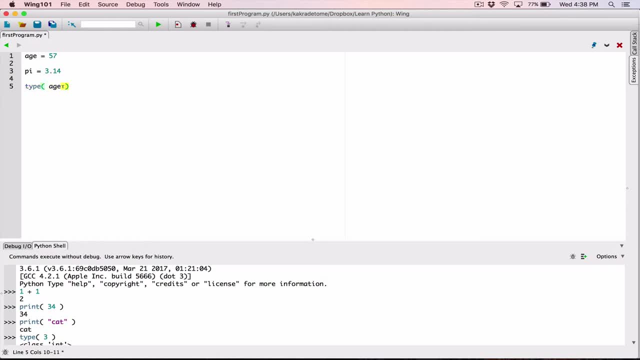 But it doesn't automatically print it. it returns it, meaning it says: okay, I've been able to figure out The type of data age is. I am, I am, I'm giving it to you. okay, privately, but you can decide. 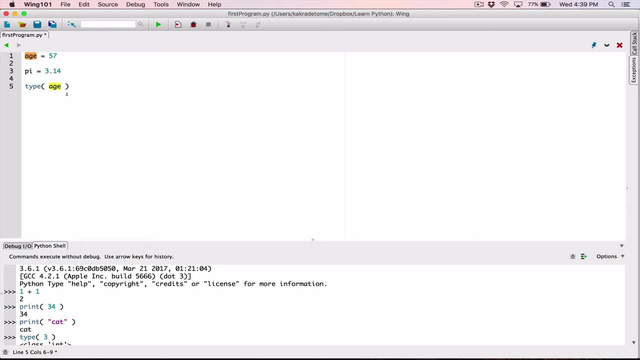 to show it. if you want, You can decide to print it if you want. It's what's called returning. It just returns to you. it returns to you the answer. Now, the interactions pane will just tell you the answer. right, But then it wouldn't print out. 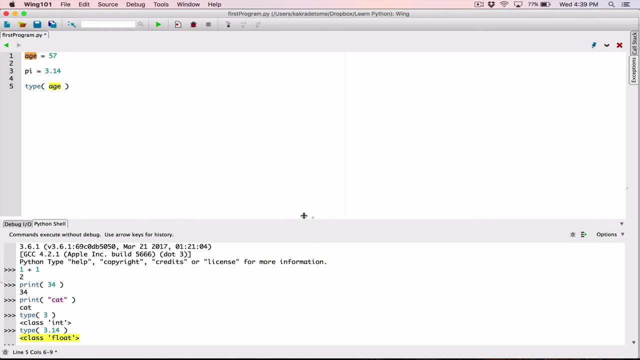 Sorry, sorry, sorry. The interactions pane will, will print some. I mean sorry, the interactions pane will figure out the answer And then, and then print it out, because that's how it's designed. But then the script mode wouldn't print it out automatically because the type function. 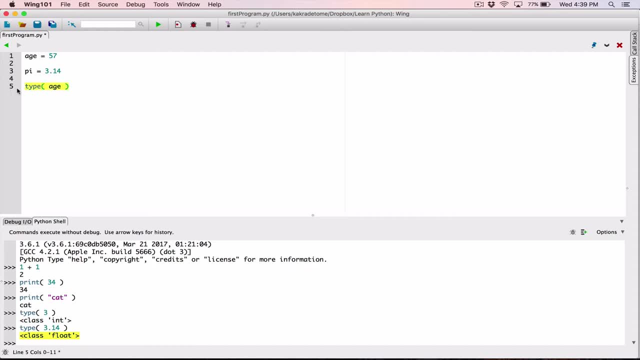 the way it works is. the way it works is it determines the type of data this is and returns it. It doesn't print it out automatically. So if I run this program, nothing happens, because it's it has determined the type of data age is and it's returning it. 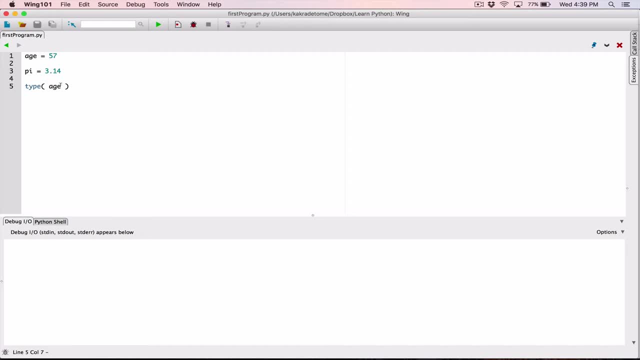 It's like it's standing in front of me. you know stretching, you know stretching, stretching its arms to me with an answer. So I have to take the answer right and do something with it. So we know that the print function works in such a way that we know that the print function 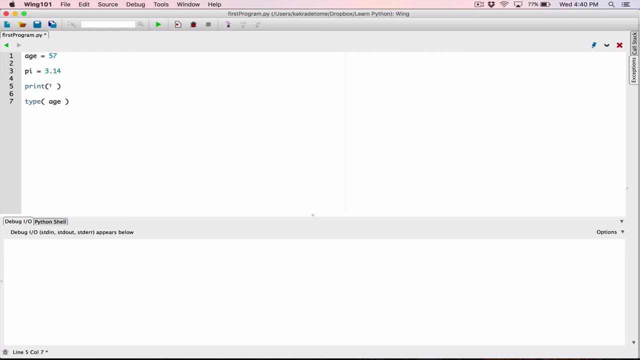 works in such a way that it takes in something here, an argument here, and print it out And we know by calling this line here it's returning, it's giving us, it's standing, you know, in front of us stretching its arms and giving us the answer, or basically the. 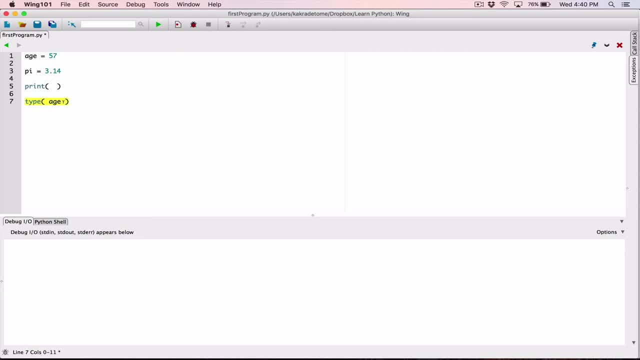 response. It's telling us: okay, this age is of type something, And so I can cut this whole line. cut it and print out what it's telling us, okay, in the parentheses. I'm going to undo Now, the print function has parentheses over here. 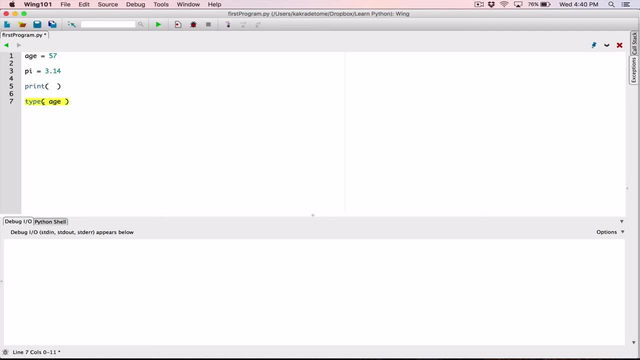 It's waiting for something to print And we know that the type function over here is kind of telling us- okay, it's kind of telling us- the type of data ages. It's not printing it out yet because you know that's not its job. 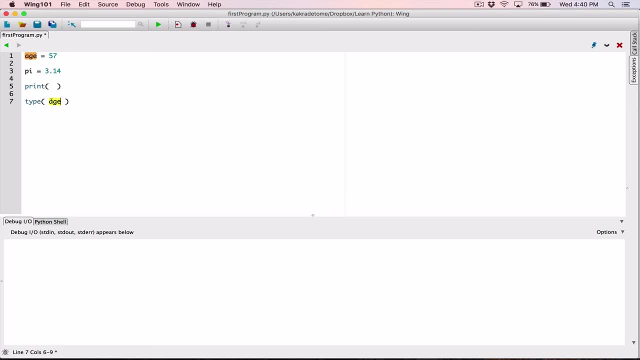 Its job is just to figure out what the type of data age is and tell you, And the print function just displays it to us. So I want to display, I want to print out the type of data ages. right Now. we'll get more into functions. 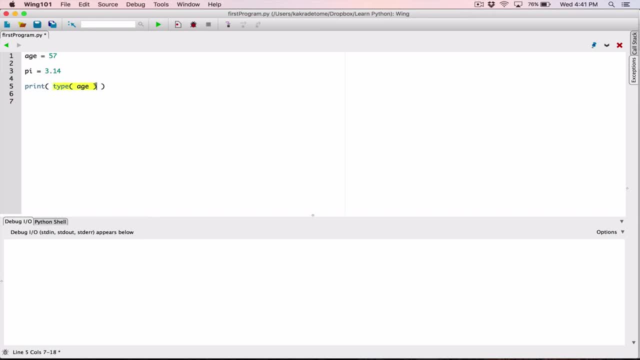 I don't even know why I kind of complicated it here. but this is just to give you a heads up of functions And we're going to cover it in the details, so don't worry too much about it. But I just wanted you to see the type function and how useful it is, you know, to determining. 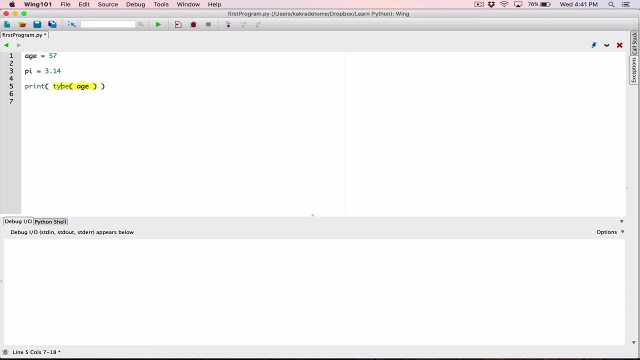 the type of data you are working with. And so when I print, Print out the type of data ages, and when I run this program, it's telling me that ages of class int. Well, basically all it's saying is that this value age, is an int over here, see. 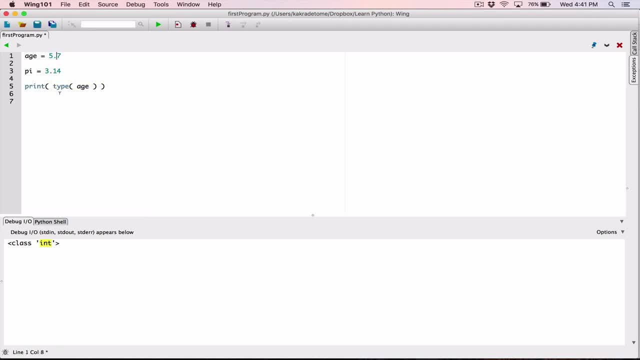 If I put a decimal in between that 5.7, make it 5.7, it becomes a float. When I run this now, it changes to a float because it's a numeric value with a decimal point. All right, so this is just to let you know of the type function.